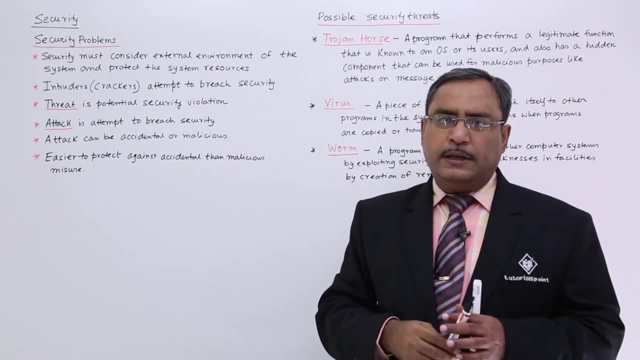 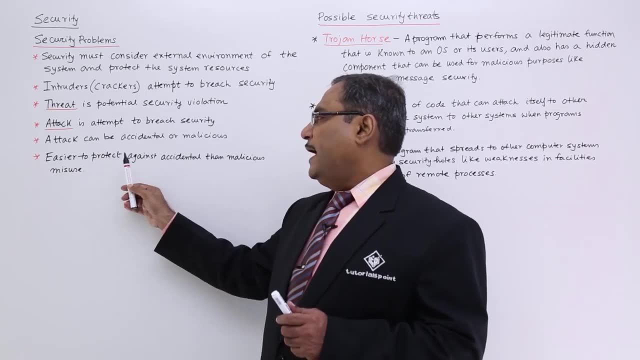 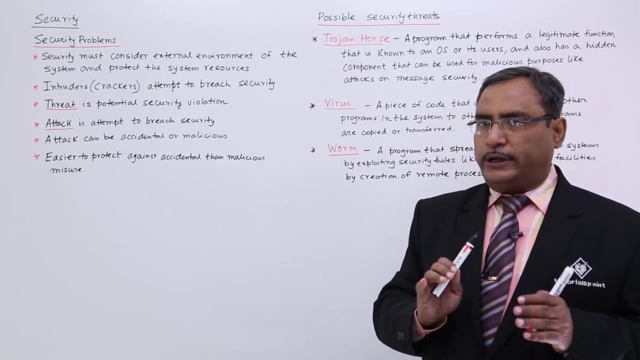 between this threat and attack. Attack can be malicious or attack can be accidental, but it is easier to protect. It is easier to protect against accidental than malicious misuse. Accidental misuse can be protected, but malicious misuse is difficult to protect compared to this one. 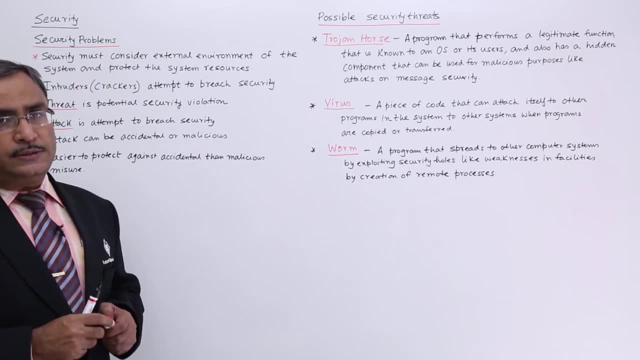 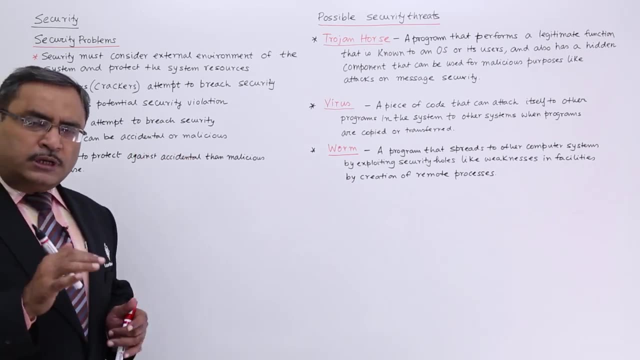 Now, here we are going for possible security threats. What are the possible security threats? I have listed 3 of them. One is your trojan horse. Now, trojan horse will be known to the user. Trojan horse. one application which is known to the westernised and westernised. to the westernised and westernised. That is why the trojan horse is known to a lot of the westernised ones. So most of the trojan horses. you have seen a trojan horses. You have seen a trojan horse or a trojan horse. Now the trojan horse. what kind of a trojan horse? 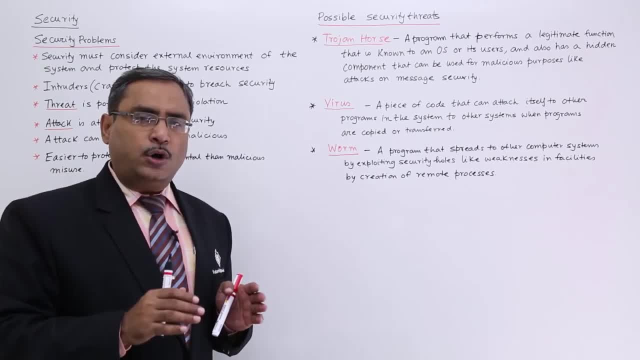 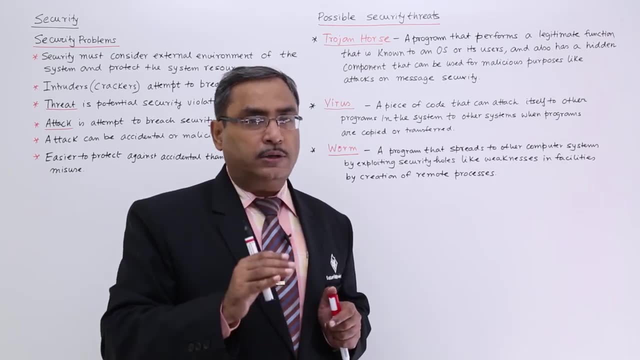 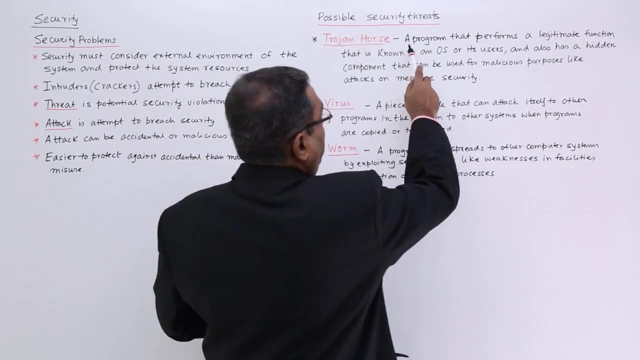 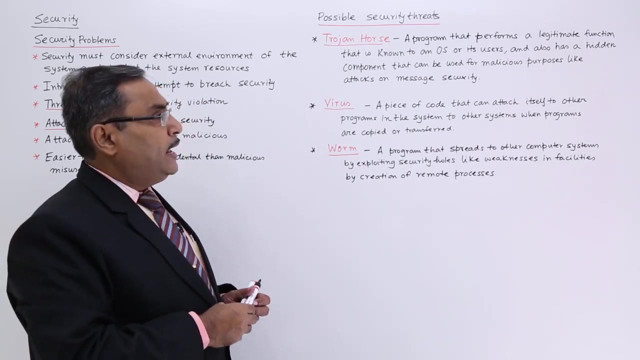 also- and it is supposed to do- some legitimate operations. these operations are legitimate operations, but behind that legitimate operation it will do some malicious activities, and that is known as the trojan horse, a program that performs a legitimate function that is known to an os or to its users and also has a hidden component. that is the main issue- also has 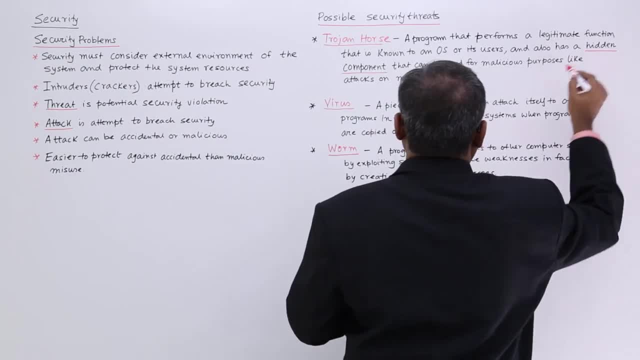 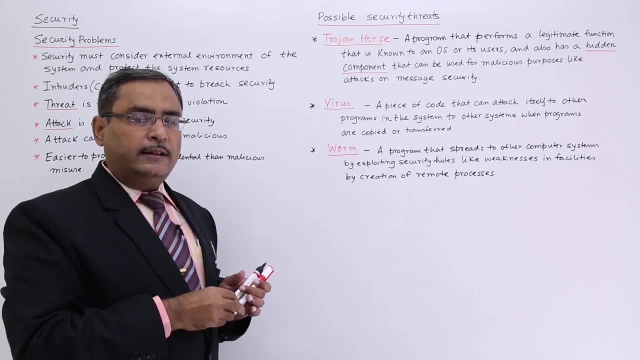 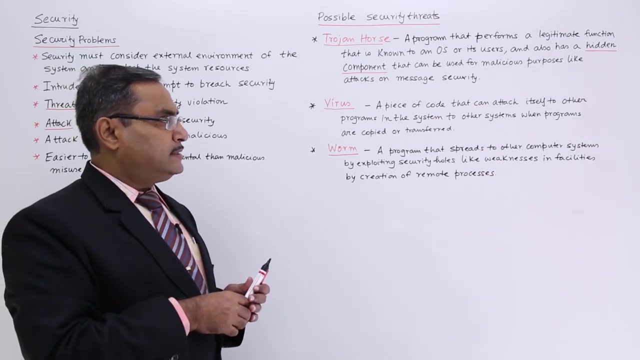 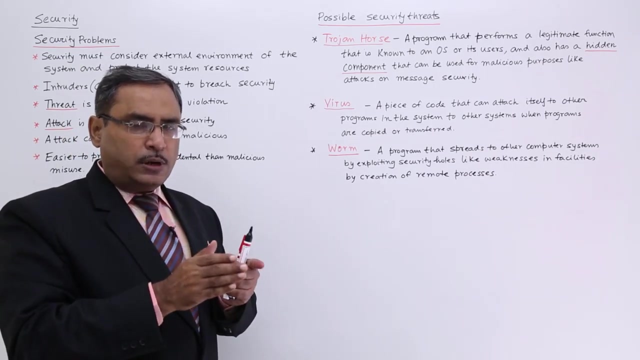 a hidden component that can be used for malicious purposes, like attacks on message security, and that is known as the trojan horse virus, a piece of code that can be attached itself to other programs in the system. so virus is a code, piece of code which will get attached. 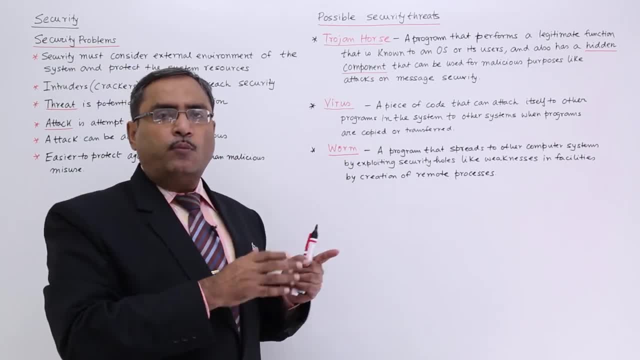 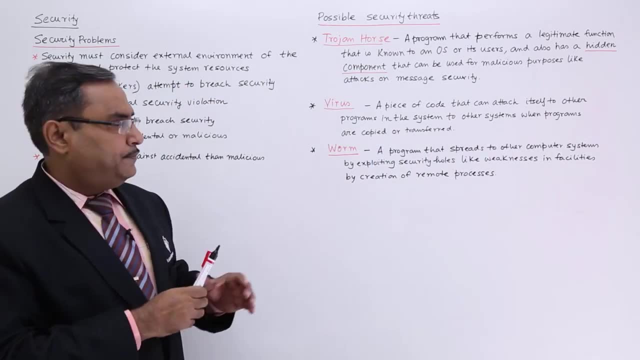 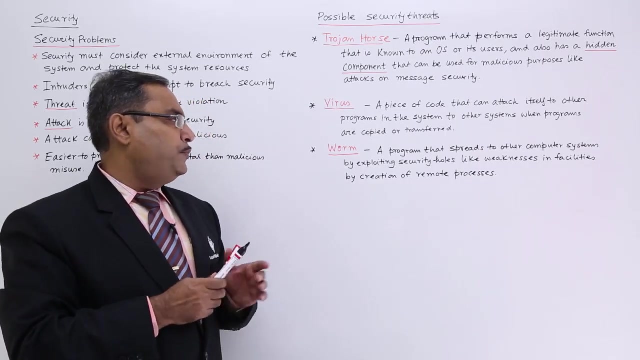 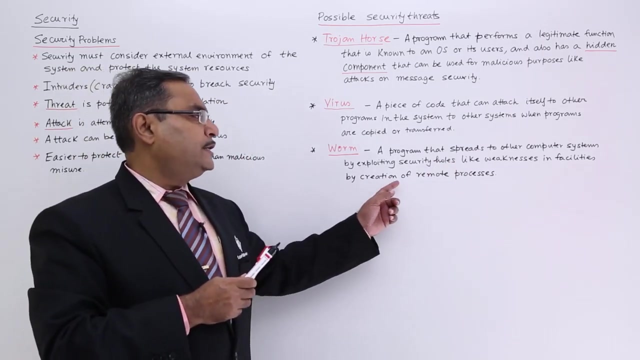 with other applications and when you are transferring that application from one system to another system. the virus will also propagate when the programs are copied or transferred. next one is the worm. worm is quite different from virus, a program that spreads to other computer system by exploiting security holes like weaknesses in the facilities, by creation of remote processes. 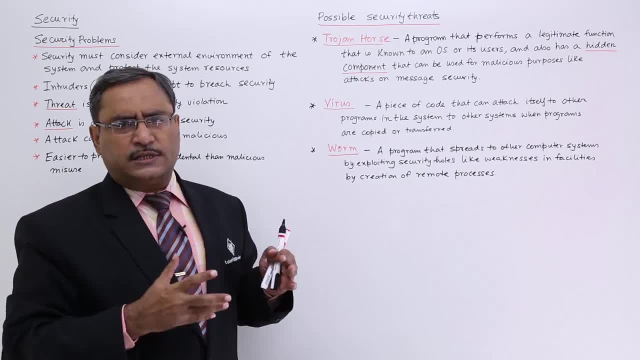 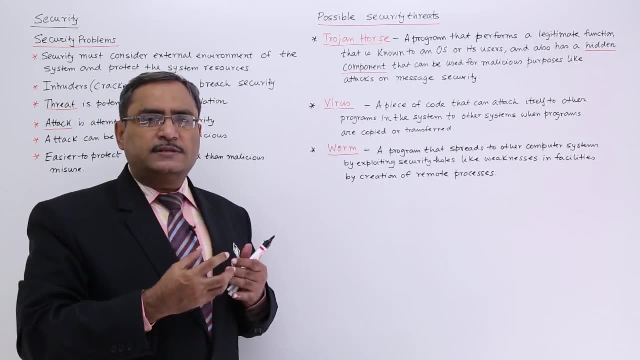 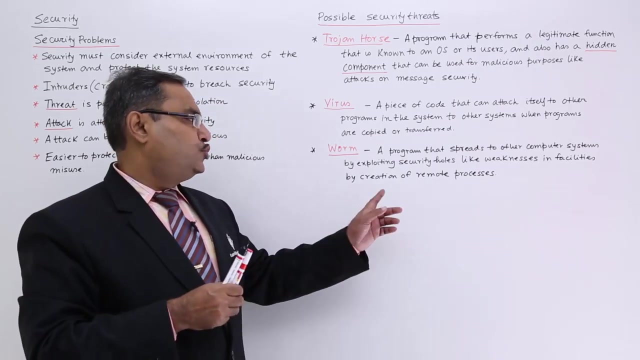 worms will always go on replicating itself and so many processes, so many threads, will get generated in the memory. So, as a result of that, my core application will be suffering from lack of memory. so my application will be going very slow and worms will go on creating so many remote processes.